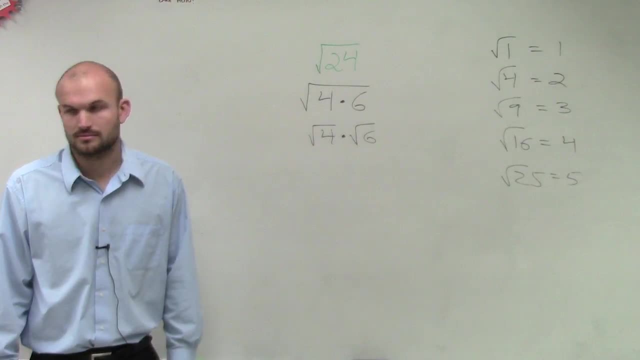 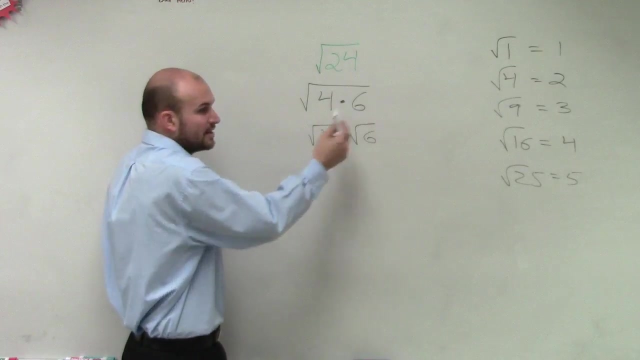 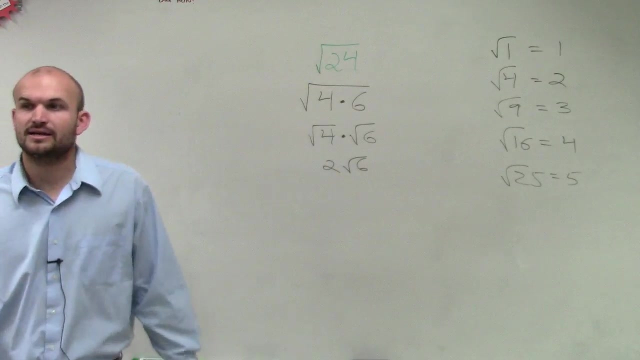 guys want me to quickly show you how that works again. Sure, So therefore, you simplify the square root of 4.. The reason why we need a square number? because, lookit, you can simplify the square root of 4, which is 2, radical 6.. So then it gets to the point where students 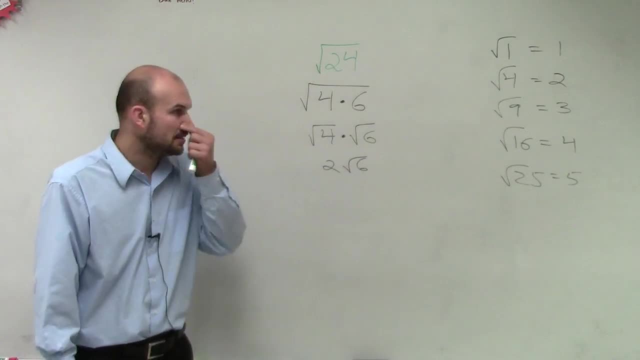 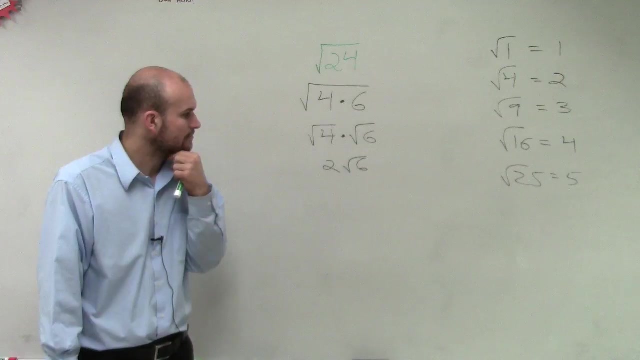 are like: well, Ms McLogan, Ms McLogan, And why can't we do? actually, this one wouldn't work. Well, 8 and 6, you can still actually even simplify This one. we wouldn't be able to. 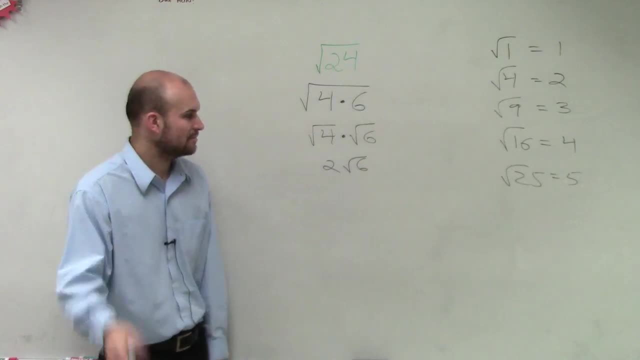 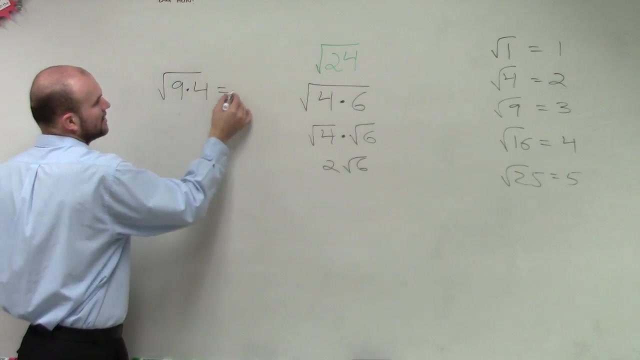 Yeah, well, you could work on 24.. I have another example, but I'll show you that, to you guys, later. The reason why this works is, let's say, I do this Square root of 9 times 4, right. 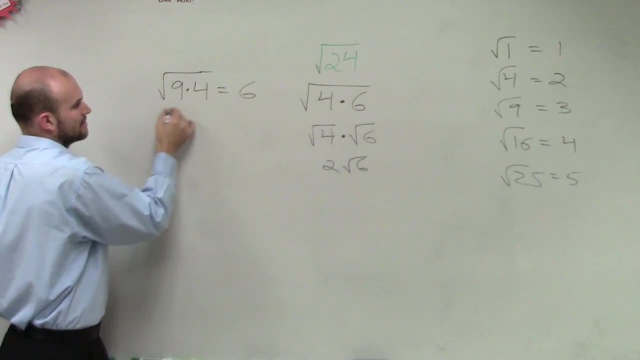 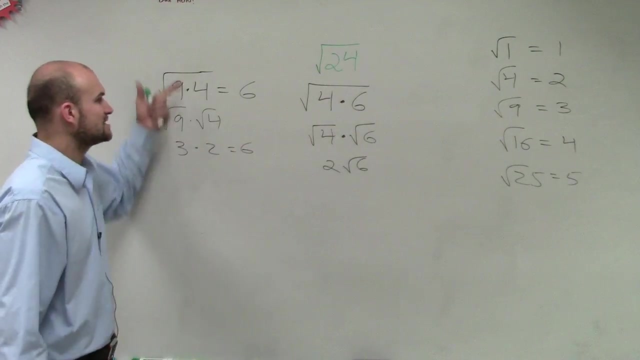 We know that answer is equal to 36.. Square root of 36 is 6.. Square root of 9 times square root of 4.. If you break it up 3 times 2 equals 6.. So that's why, when you can break up a number into the product of two numbers, 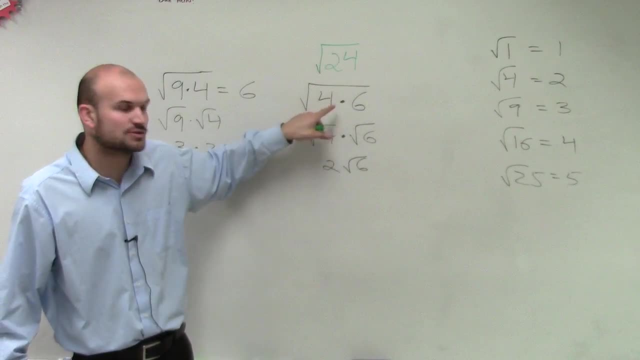 make sure that one of those numbers is a square number, Because once you have it as a square number, you can simplify it. Does that make a little more sense? Yeah, Okay, So That's not what you have to do anyway. 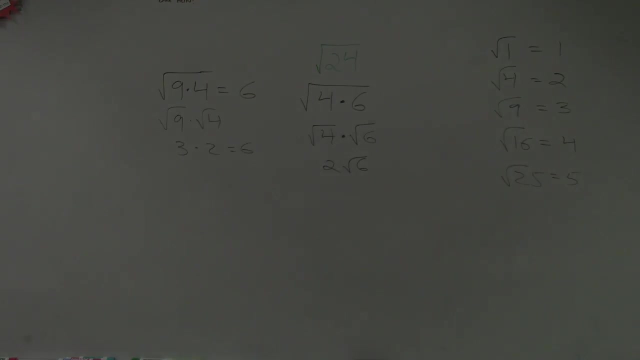 What? Nothing. That is what you have to do, But a lot of these problems.